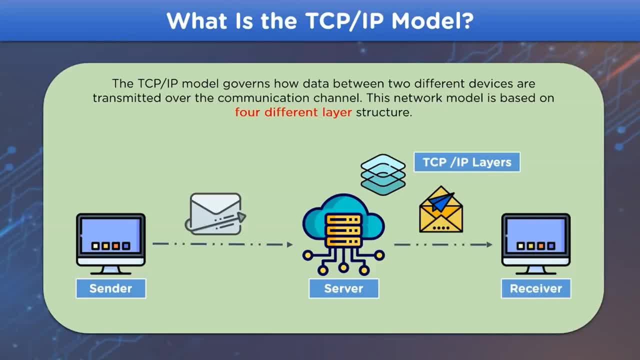 Let's begin. Firstly, we'll understand what exactly is the TCP IP model, continuing with the protocols 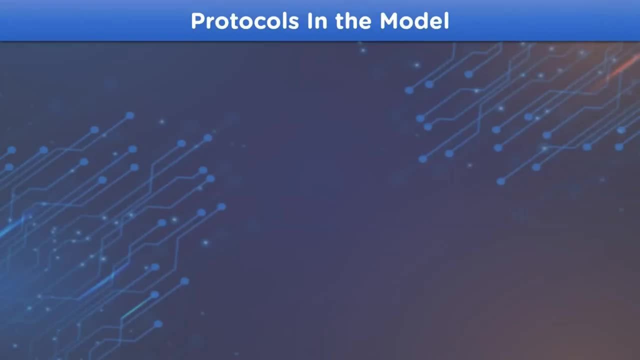 that are applied, the layer structure in the TCP and IP model. 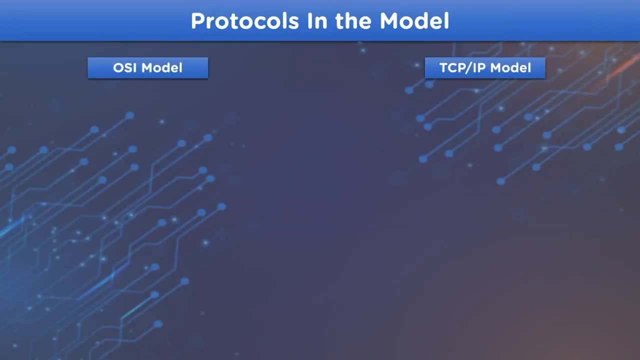 To understand the protocols that are used in the TCP IP model, we'll compare it with the OSI model. 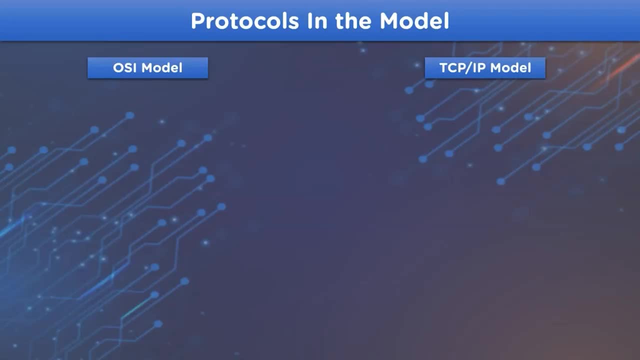 And if you want to know more about the OSI model, you can visit our video on the Simply Learn channel. Let's begin. 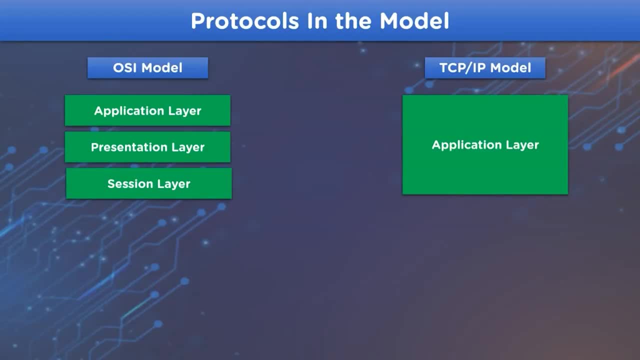 The topmost three layers of the OSI model, which are application layer, presentation layer, and the TCP IP model. 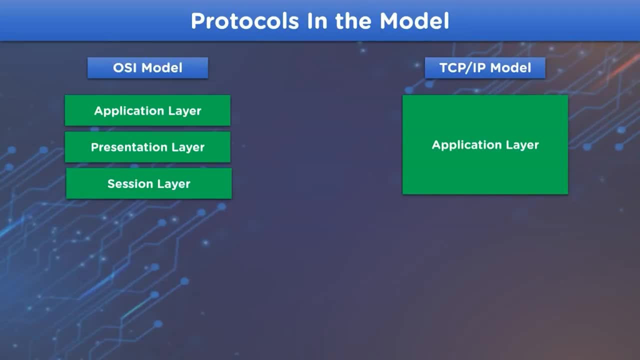 The application layer and the transmission layer collectively refers to the application layer in the TCP IP model, where they use protocols such as FTP file transfer protocol, 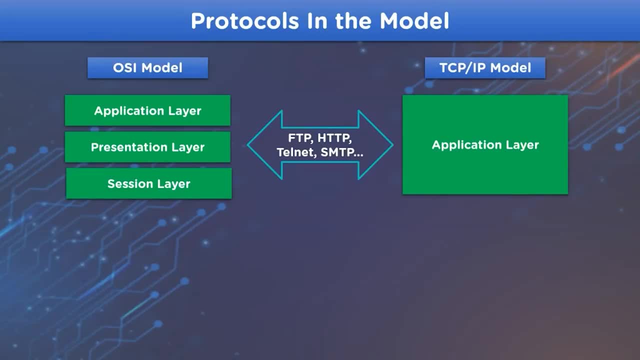 HTTP hypertext transfer protocol, Telnet, and SMTP, which is simple mail transfer protocol. 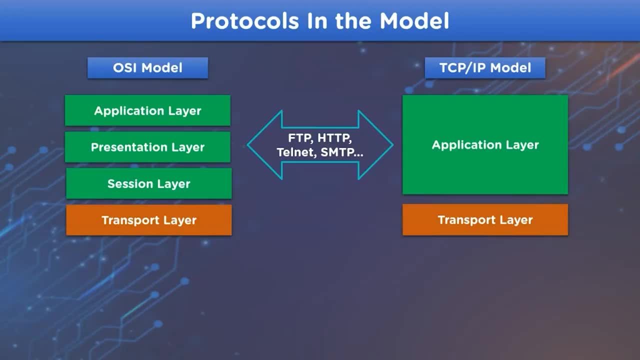 Then we have the transport layer from OSI model, which refers to the transport layer in the TCP IP model, where they apply protocols such as TCP. Transmission control protocol refers to the TCP IP model, and the TCP IP model refers to the TCP IP model. 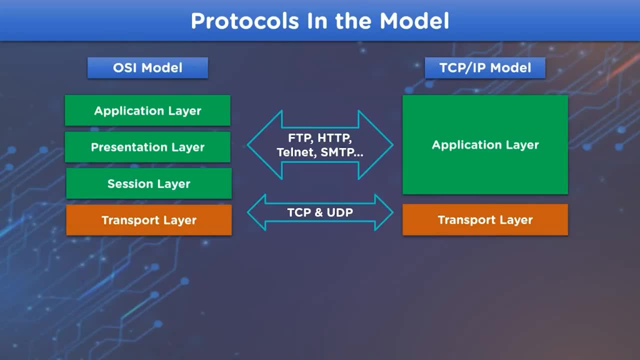 Transmission control protocol and UDP, user datagram protocol. Moving on, we have network layer from the OSI model, which refers to the internet layer 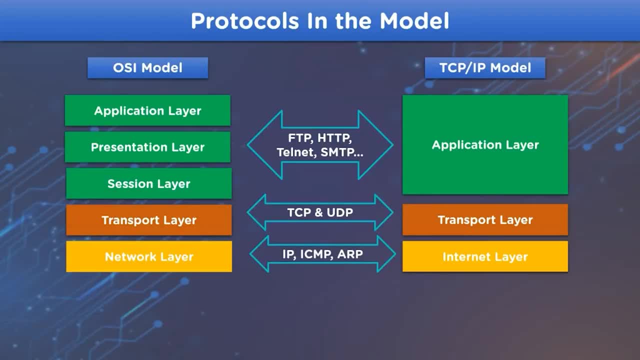 in the TCP IP model, which apply protocols such as IP internet protocol, ICMP internet control message protocol, and ARP, address resolution protocol. 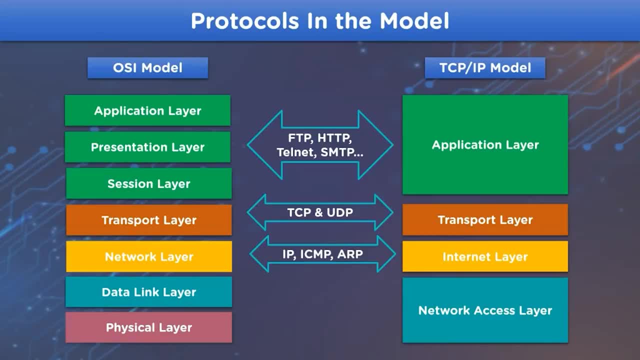 Then we have data link layer and physical layer from the OSI model, which refer to the network access layer in the TCP IP model. 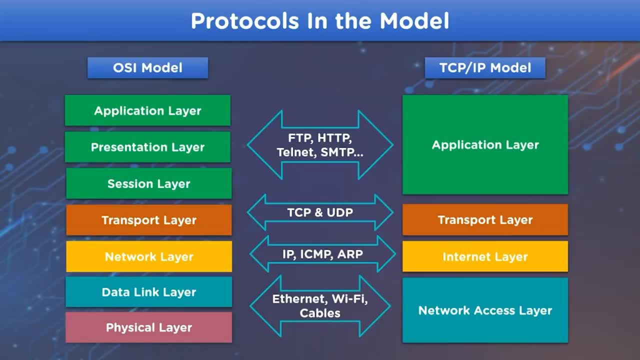 These layer doesn't exactly apply any protocol, but are connected through physical medium, which includes Ethernet, Wi-Fi, and cables. 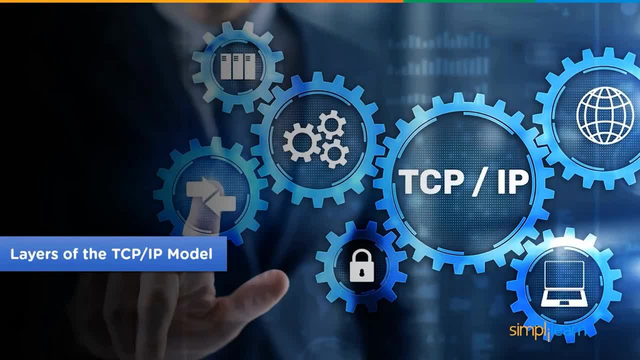 Now that we are completed with the protocols regarding TCP IP model, let's take a look at the layers in detail. 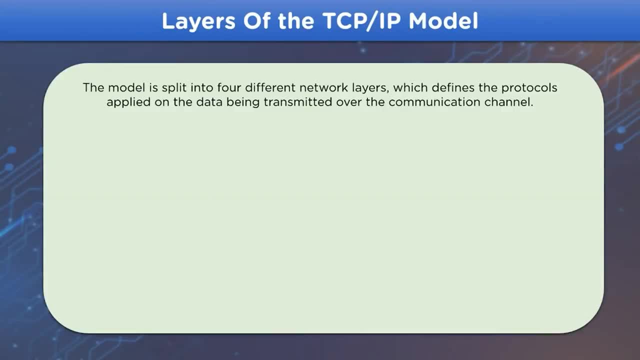 The TCP IP network model consists of different layers. Where? The application model consists of four different layers, which are application layer, transport 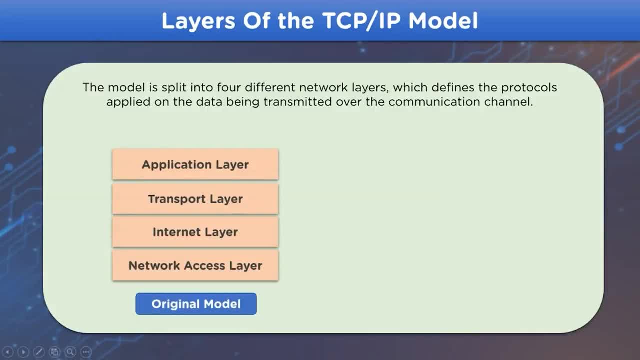 layer, internet layer, and network access layer. 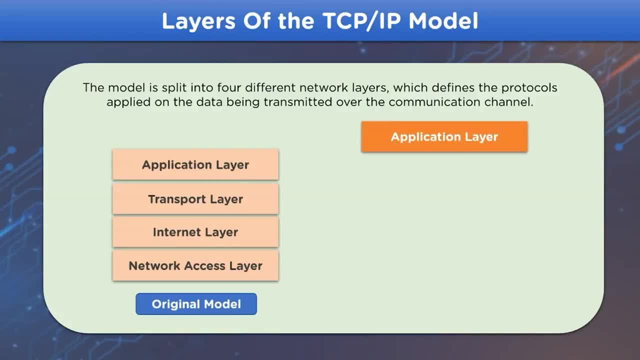 Then we have the updated model, which consists of layer, application layer, transport layer, 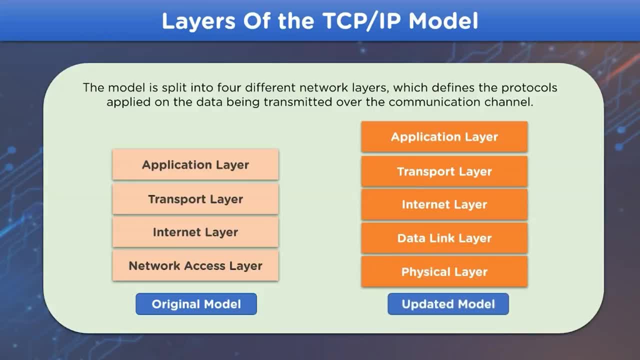 internet layer, data link layer, and physical layer. 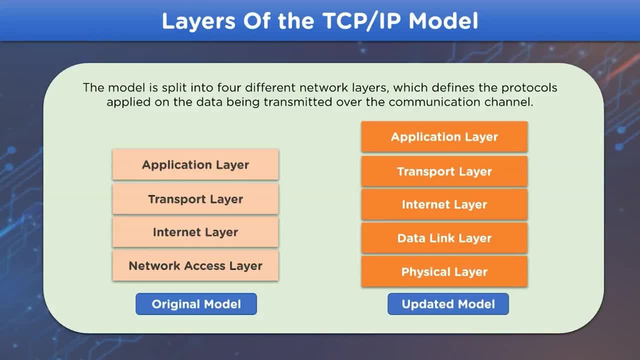 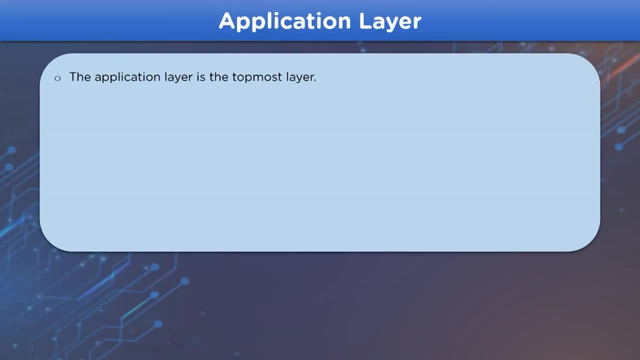 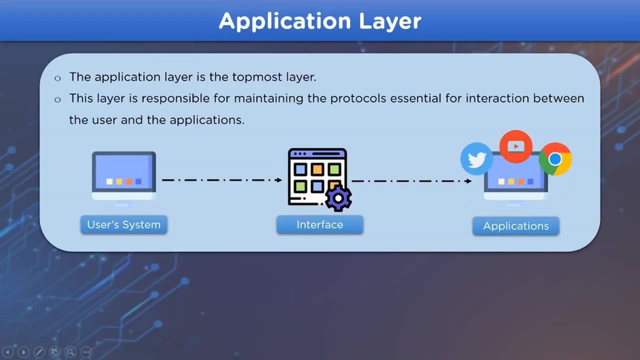 Let's take a look at the layers in detail. The first layer that we are going to know about is the application layer. Application layer is the application layer. This layer acts as an interface between the application and programs that require the TCP IP model for communication, including tasks performed by the layer, such as data representation for the software application that are executed by the user, and then forwarded to the transport layer. 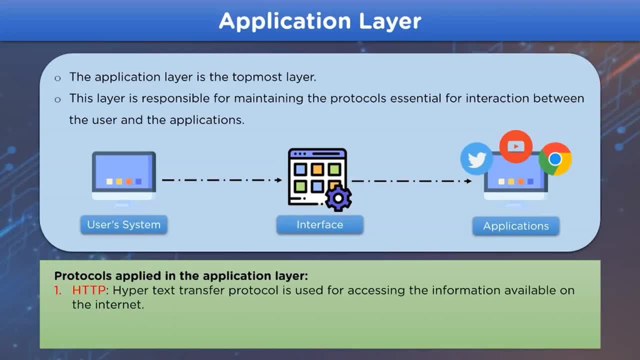 The protocols applied by these layers are, HTTP, hypertext transfer protocol, which is used to access information available to the user. Then we have the communication layer. This layer acts as an interface between the application layer and the transport layer. 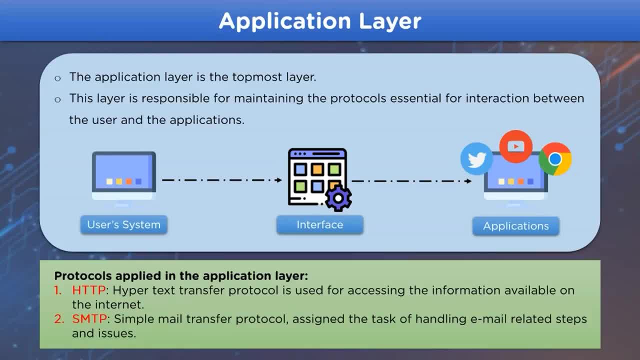 Then we have SMTP, simple mail transfer protocol, which is used to access email related tasks. 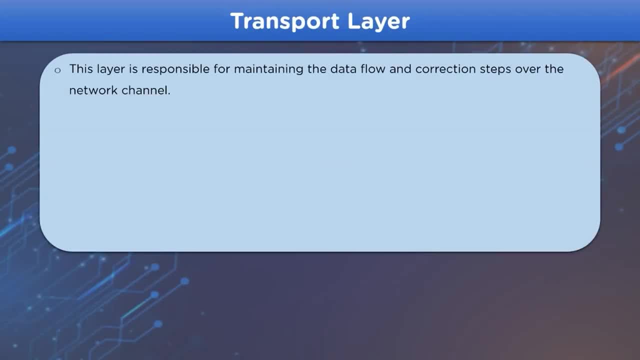 Moving forward, we have the transport layer. This layer is responsible for establishing connection between the sender and the receiver device. 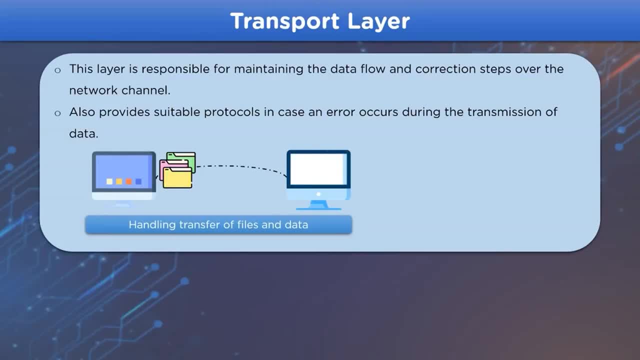 This layer performed the task of dividing the data from the application layer into packets, where they are used to create sequences, which are then transferred over to the destination device. 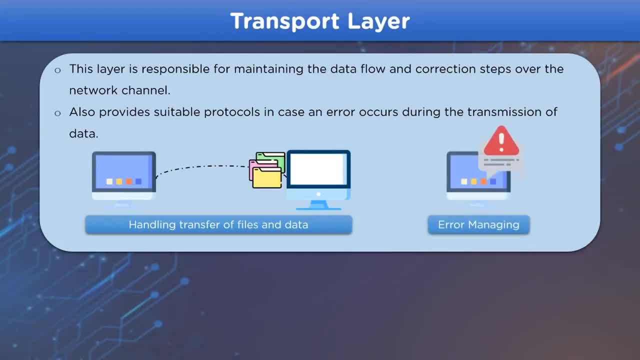 It also performs the task of maintaining the data, that is, to be transmitted without error and controls the data flow rate. 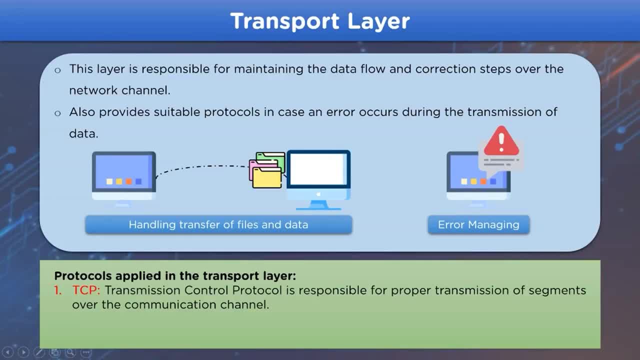 The protocols that are applied in the transport layer are, TCP, transmission control protocol, which is responsible for transmission of segments over the communication channel. Then we have UDP, user datagram protocol, which is responsible for identifying error in the data. 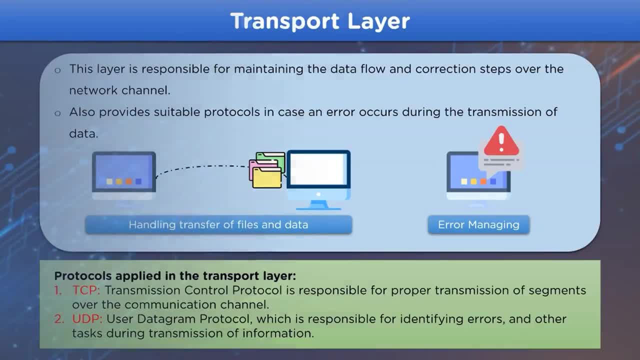 It also performs the task of identifying error in the data flow rate, which is responsible for identifying error in the data flow rate. 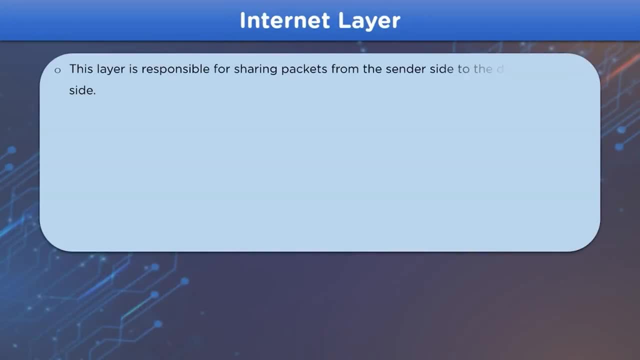 Moving forward, the next layer is the internet layer. This layer is responsible for the transmission of data over the network channel, that is, they provide a proper route for the packets to be transferred over the communication channel. The protocols that are applied by this internet layer are, IP protocol, which is the internet protocol. 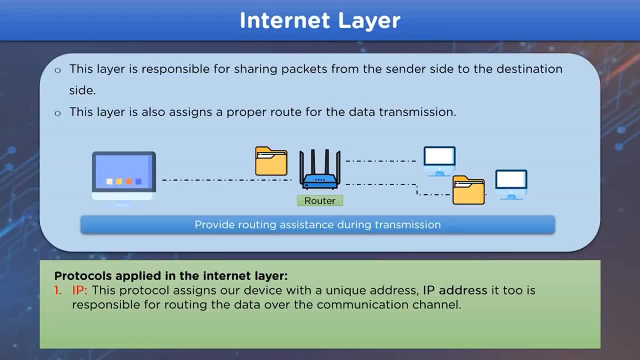 This protocol assigns a unique address to a physical system, so that it can be identified on the internet. 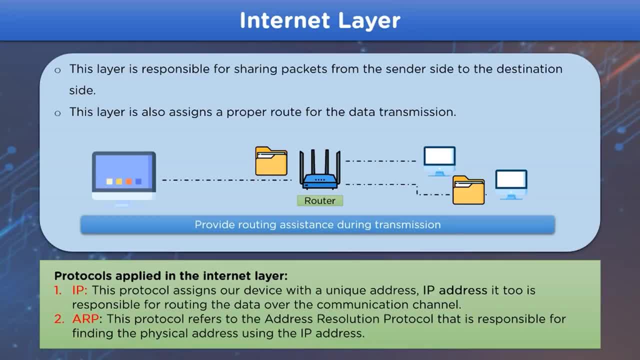 Then we have ARP, address resolution protocol. This protocol is used to find the physical address of the system using the internet protocol address. 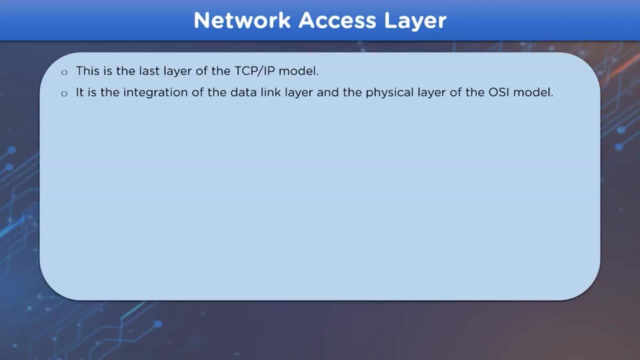 In the end we have the network access layer. This layer is a combination of data link layer. This layer is a combination of data link layer and network access layer. This layer is a combination of data link layer and network access layer. This layer is a combination of data link layer and network access layer. And it is the same physical layer from the USM model, where it is responsible for maintaining the task of sending and receiving data in raw bits. 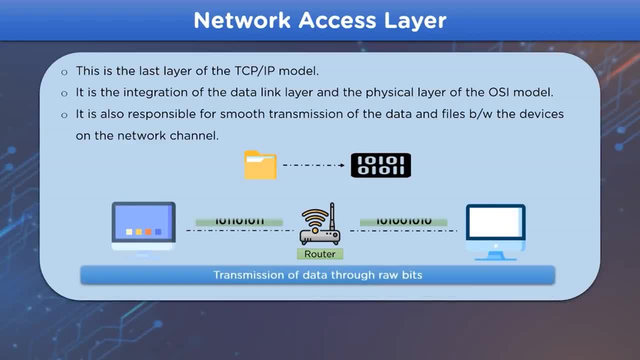 The raw bits are transferred from the sender side to the receiver side in the format of binary digits, which are zeros and ones. 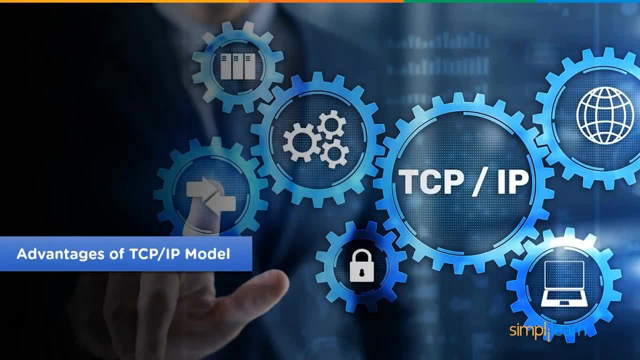 Let's move on with the advantages of using the TCP IP model. 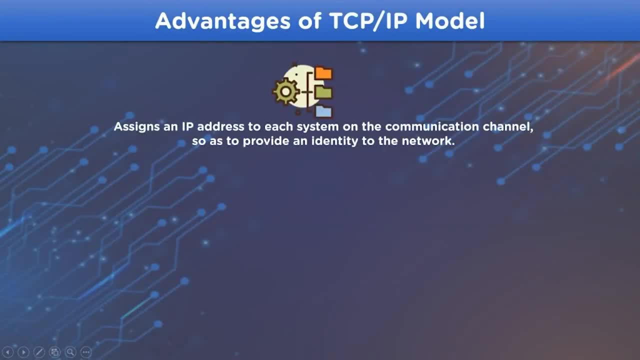 Let's move on with the advantages of using the TCP IP model. assigns an IP address to each of the system that is available on the network channel so that they can be identified on the internet. Then they are also responsible for enacting different protocols 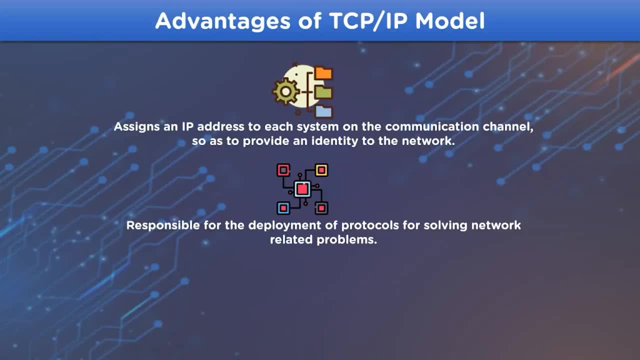 on the data that is to be transmitted over the communication channel. The TCP IP model also enables the user and the system to access different format of data over the communication 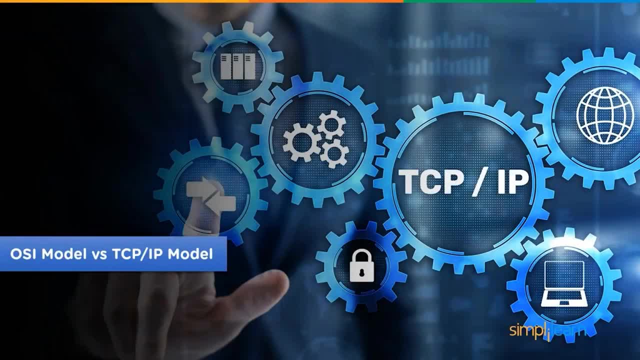 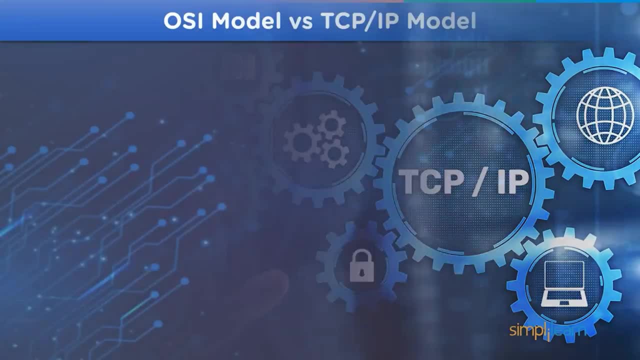 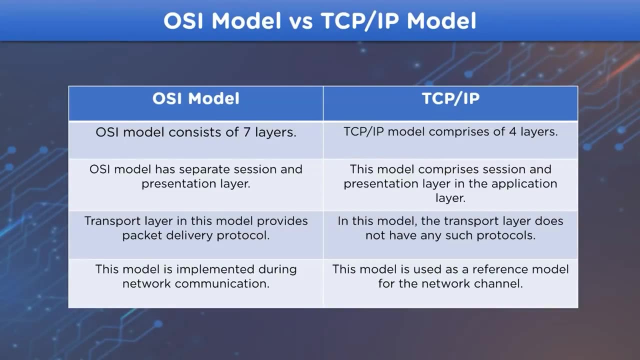 channel. Now let's take a look at the last topic for this session which is the OSI model versus the TCP IP model. On comparing both of the network models we get the OSI model consists of seven 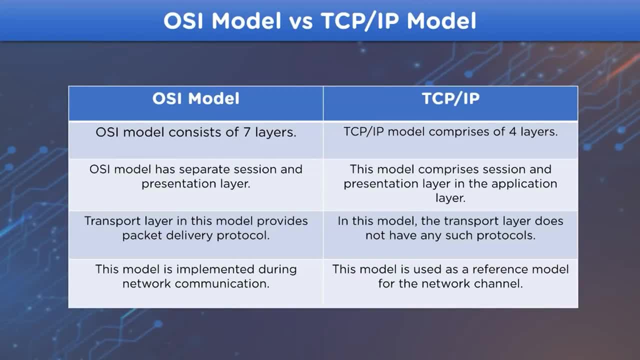 different layers whereas the TCP IP model comprises of four different layers. The OSI model has separate session layer, presentation layer, whereas the TCP IP model comprises of a single application layer. The transport layer in the OSI model provides packet